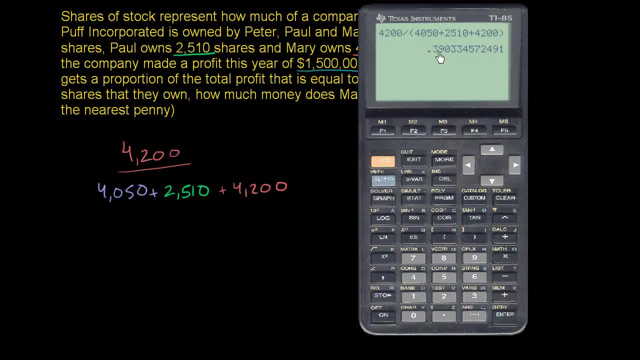 And so Mary should get 0.39 of the profit. Or if we talk about it in terms of percentage, it would be 39% of the profit. So this right over here is 0.390.. Actually, let me just leave it like that. 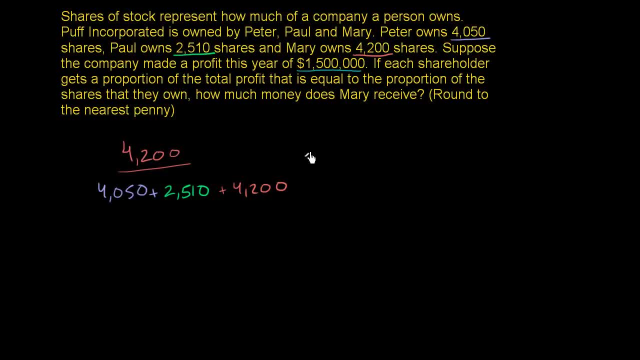 So this is approximately equal to 0.39.. And so if we want to figure out how much profit she gets, she gets this much times the total profit. So Mary gets 0.39.. And this is the exact quantity right over here. 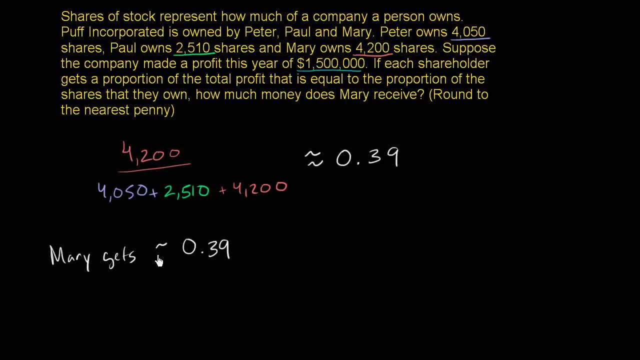 0.39 is the approximation, So approximately 0.39, this little squiggly equal sign is how I say approximately. She's going to get 0.39 times the total profit, which is $1,500,000.. 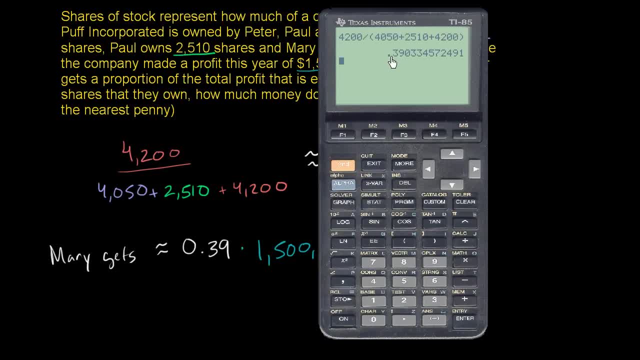 And so let's go back to our calculator. And so we said: approximately 0.39.. This is the exact value. I can get that exact value again, at least in this calculator, by saying second answer. This literally means the previous answer. 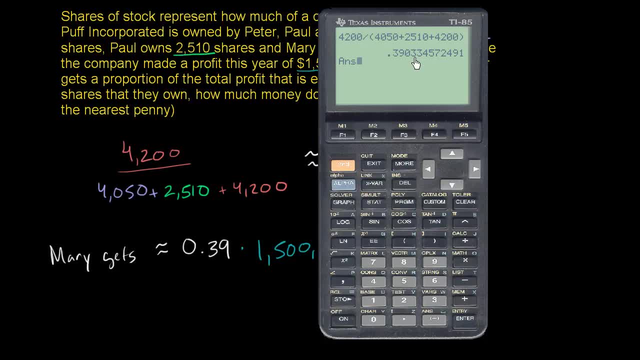 So this is literally this number right over here: 0.390334, whatever, So this is the exact quantity times $1,500,000.. One, two, three, There we go, That's $1,500,000.. 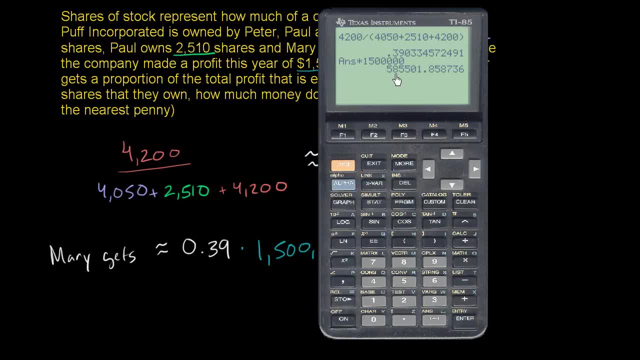 Got to make sure I have the right number of zeros there And that gets us $585,501. And we need to round to the nearest penny And $0.86.. So let me put that someplace where I can see it. 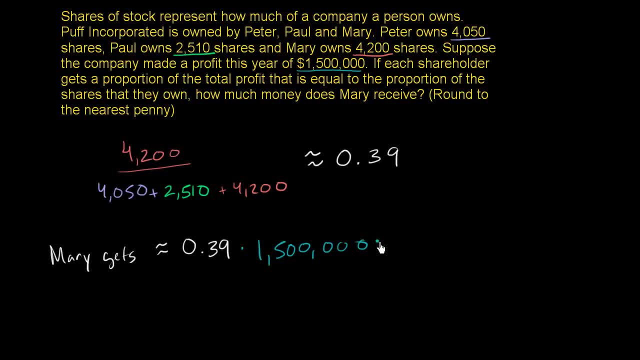 So this is going to be equal to $585,501.. And if we round $0.86.. So not bad for one year for Mary. She should be able to live quite well just on her dividends from Puff Incorporated.